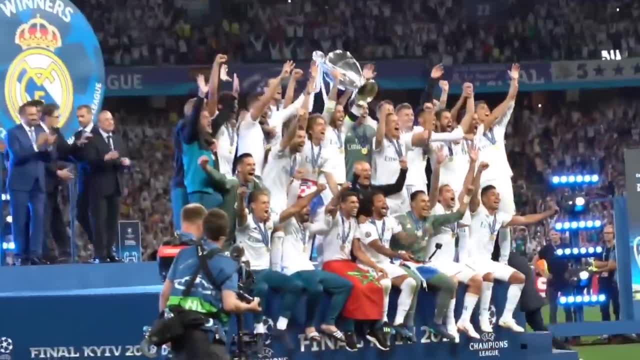 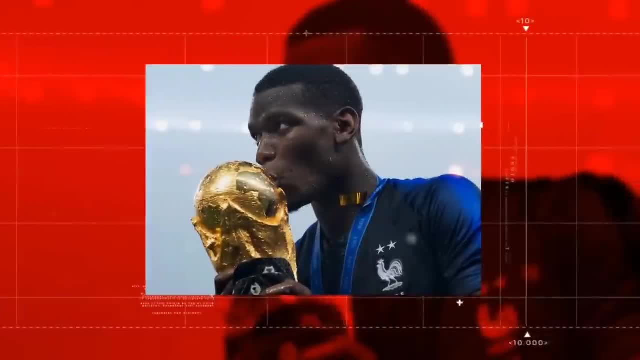 Most footballers will tell you winning trophies is all about pride and prestige, but the truth is many of those trophies have insane value on their own, And it's always so good to have your hands on the most valuable silverware. Have you ever wondered how much? 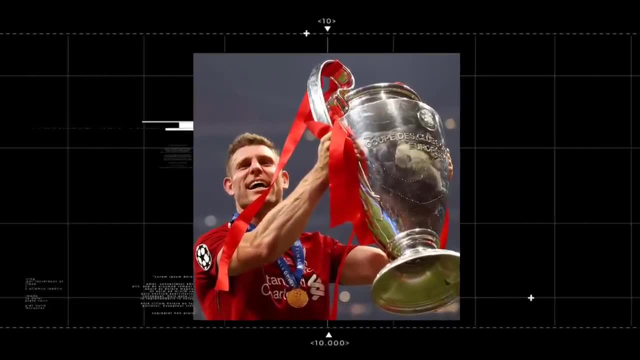 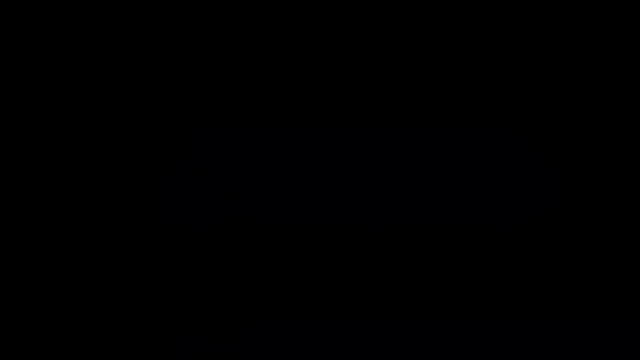 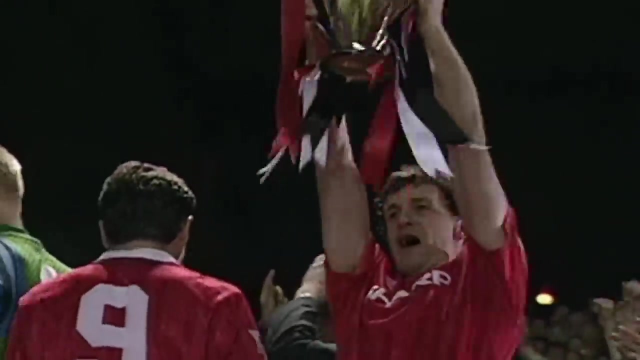 some of these trophies are worth Hundreds of thousands of dollars, Millions. Well, we'll find out in this video, as we count down the 10 most expensive trophies in the world. Number 10. The Premier League Trophy. Many players, managers and even fans want to win the Premier League trophy, at least. 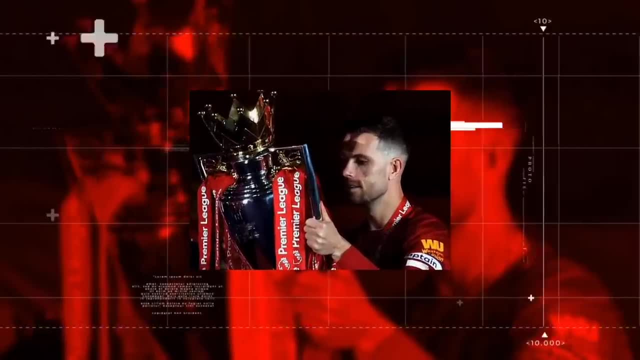 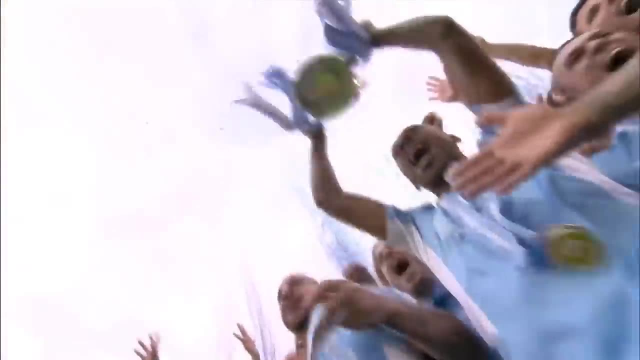 once in their careers. Many will argue that it's the toughest league title to win, and that alone makes it insanely valuable. But apart from the prestige that comes with winning the title, the Premier League trophy on its own is a pretty expensive piece of silverware. 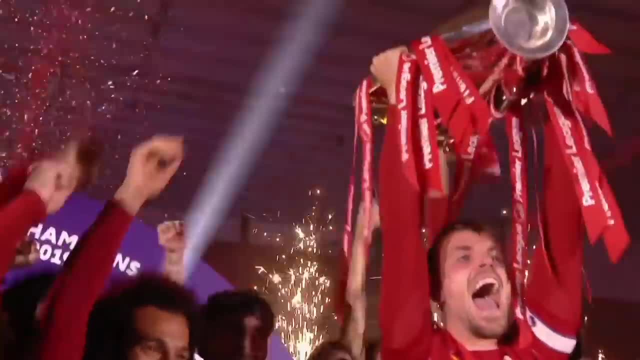 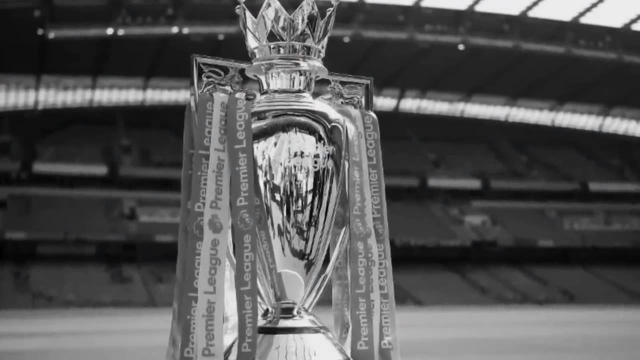 The trophy is made with malachite silver and gilded silver and is valued at $10,000.. But, as you'll later find out, it's not even close to being the most expensive league trophy, Number 9.. The UEFA Champions League Trophy. 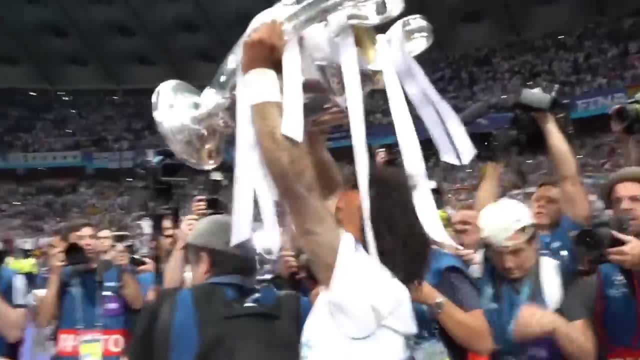 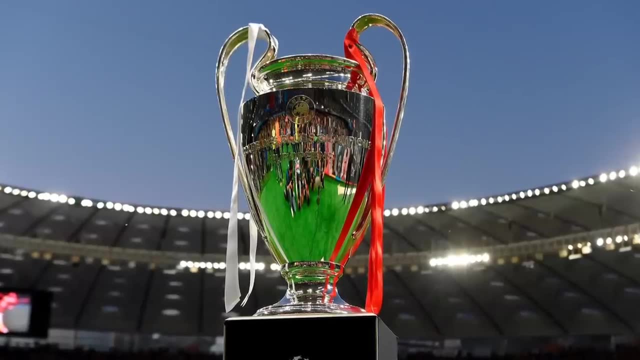 The Champions League is the zenith of European club football, and so it's not surprising that the trophy to be won is a really valuable one. The Big Ears, as it's fondly called, is 74 centimeters high and 11 kilograms heavy. 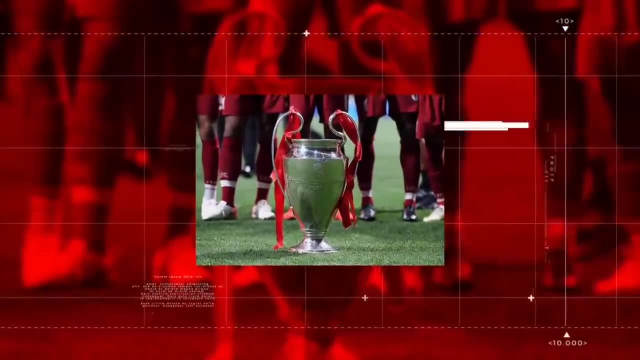 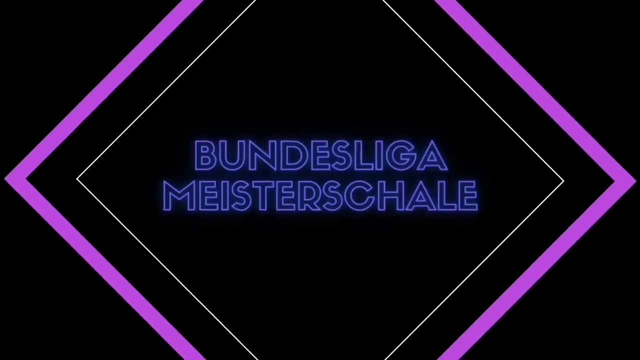 and it's made with pure silver. The UEFA Champions League Trophy is worth $15,000.. Number 8. The Bundesliga Meisterschale. The Meisterschale, which translates to Champions Bowl, is the name of the trophy given to teams. 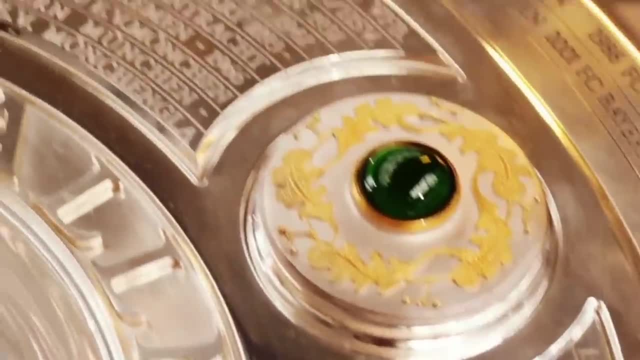 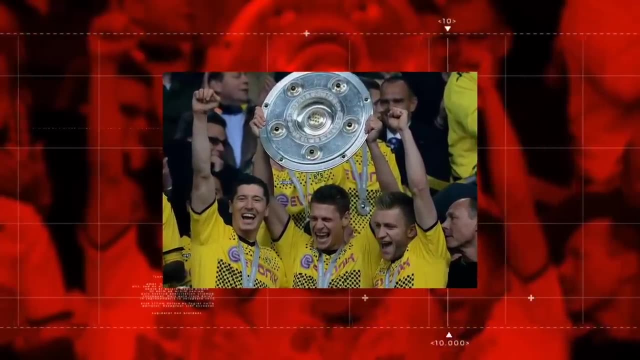 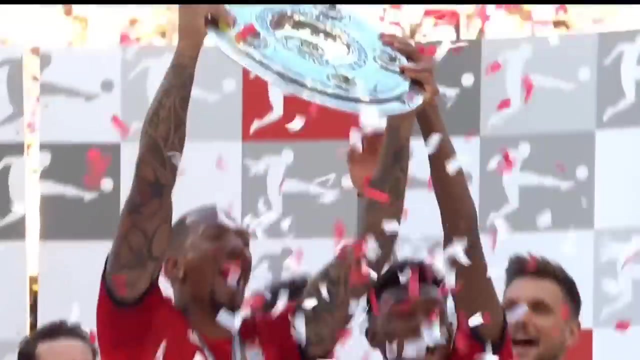 who win the German Bundesliga. The trophy has the names of all the winners since 1903 engraved on it and, as a result, it has had to be enlarged on two different occasions, in 1981 and 2009.. The current size is said to have enough space for winners' names. 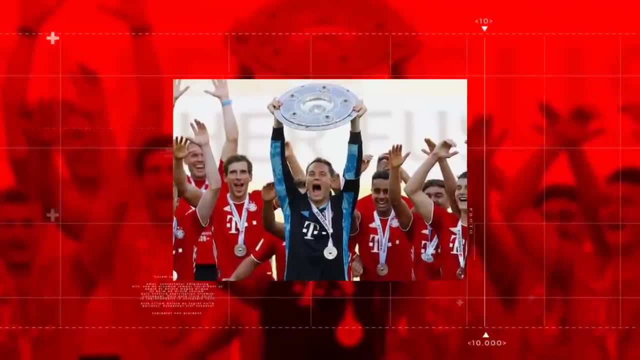 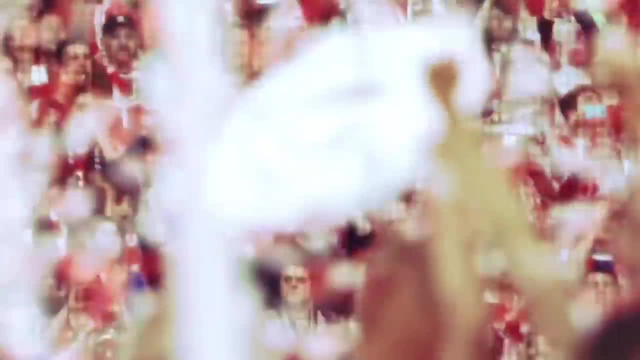 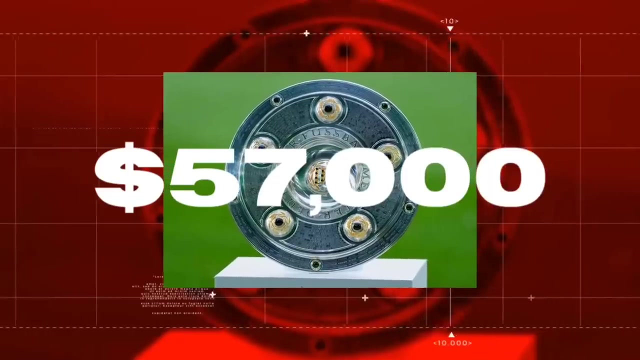 until 2026,, but from the looks of things, that's only going to continue to be one name. Anyway, the Meisterschale replaced the Victoria which got lost during World War II and has been awarded since 1949.. The Bundesliga Meisterschale is insured for 50,000 euros, That's a little more than $57,000. 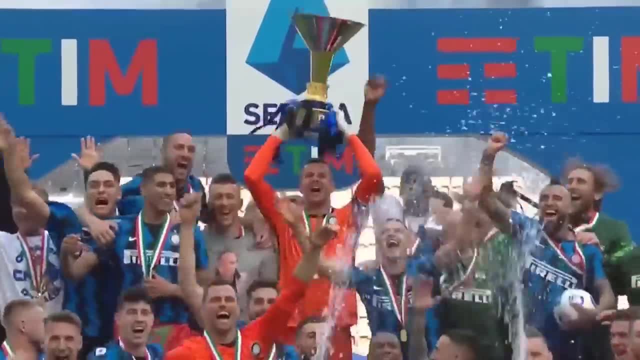 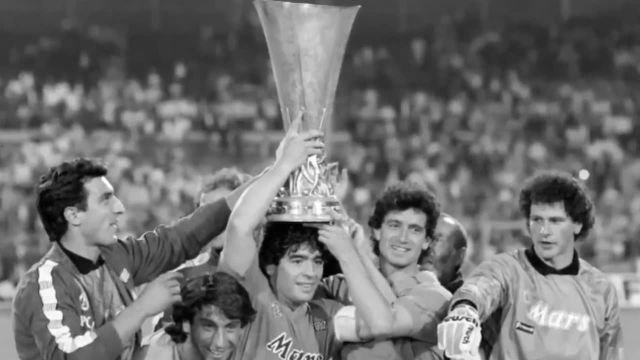 Number 7. The Scudetto. This is the trophy given to the winner of the Italian Serie A. The Scudetto was created way in the 1920s as a little decoration to be worn by the winners of the Italian top flight Genoa. 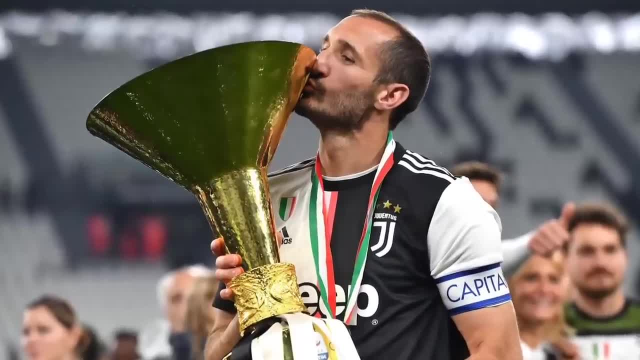 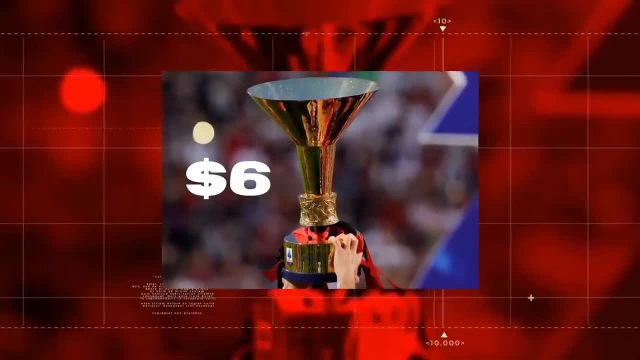 became the first team to wear it. The trophy is funnel-shaped, with a soda-like base and a gold ring. It's 8 kilograms heavy and 58 centimeters tall, and it's valued at $66,000, making it the most expensive league trophy in the world. Number 6. AFCON Trophy. The current Africa Cup of Nations trophy is the third of its kind, first awarded to Cameroon in 2002.. It's a gold-plated trophy with a ball on the top. On the ball is an engraving of the map of Africa Designed in Italy. the current AFCON trophy. replaced the African Unity Cup, which was last awarded in 2000.. It is valued at $150,000.. Number 5.: The Ballon d'Or Trophy. The Ballon d'Or trophy is the only individual trophy on this list today and it ushers us. 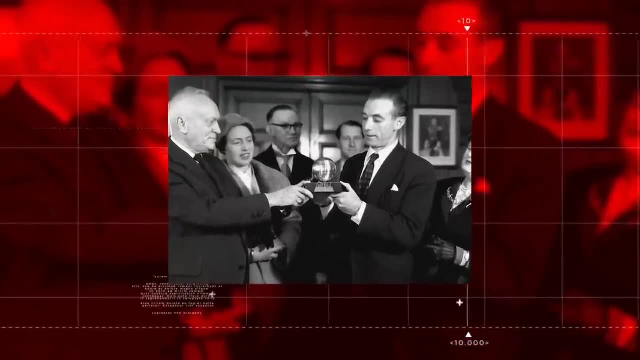 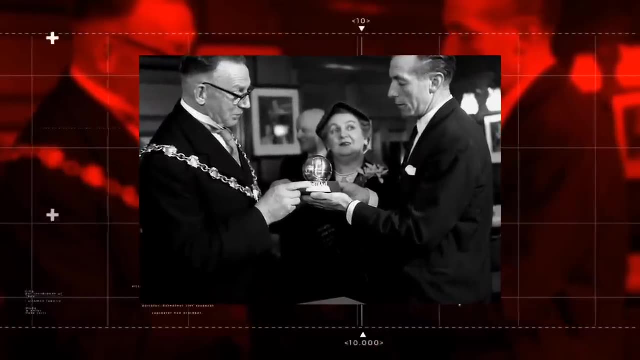 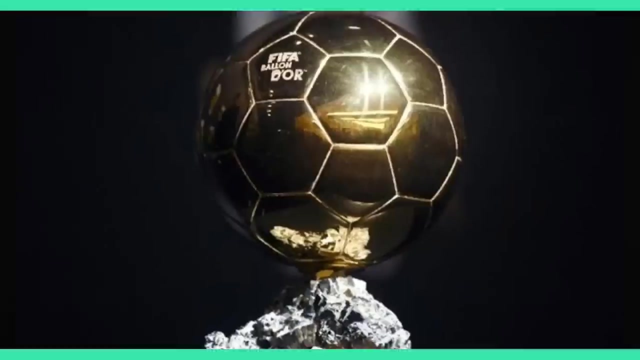 to our top 5.. The trophy, which was first awarded in 1956 to the best European player in the year under review, has grown to be an award for the outright best player in the world, which is now being awarded to the best performing player in both the men's and women's games. The trophy is: 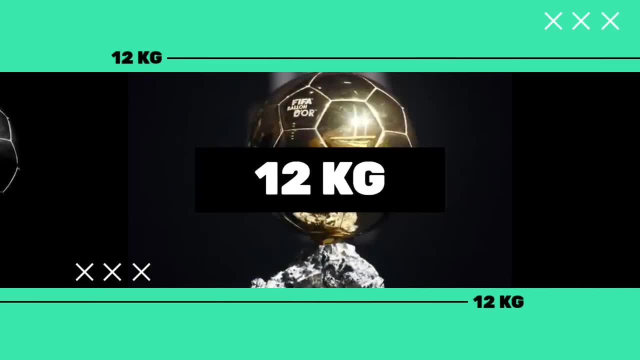 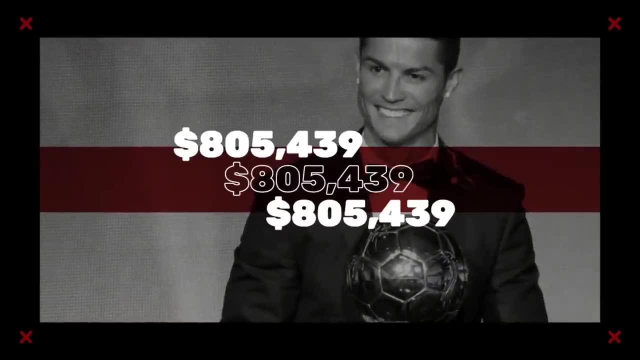 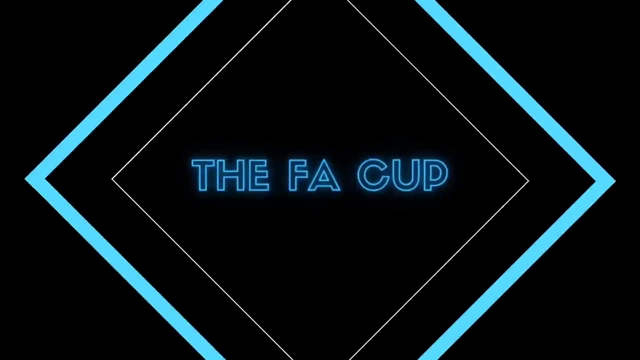 made with pure gold and it weighs about 12 kilograms. A single Ballon d'Or trophy is valued at $805,439.. Number 4. The FA Cup. Winning the FA Cup might not be as big a deal as winning the Premier League, but the trophy. although smaller, is actually more than 100 times the value of the Premier League trophy. The FA Cup trophy is made with sterling silver and it is valued at $1.18 million. It took designers 250 hours to develop this trophy, which stands at a height of 61.5. centimeters and weighs 6.3 kilograms. But wait a minute. the FA Cup trophy is worth over a million dollars and it doesn't even make the top three most expensive trophies in the world, Wow, So why don't we just go straight and see which trophies make up the top three? 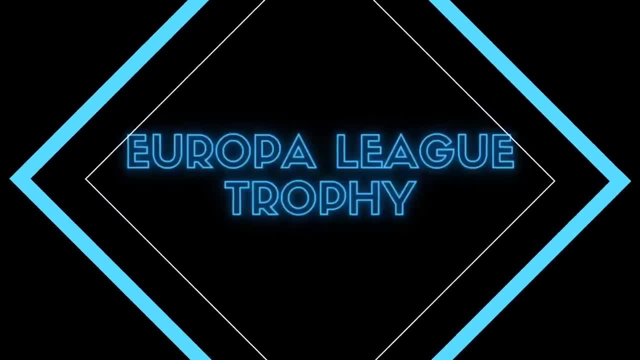 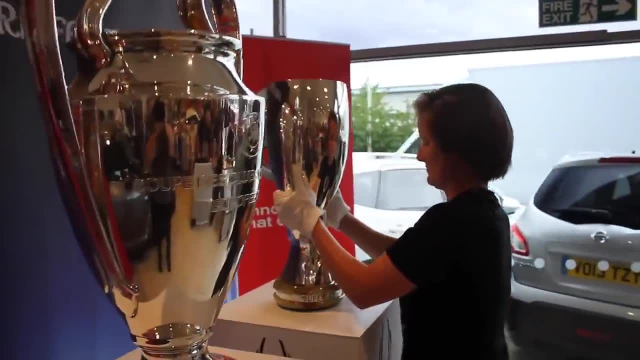 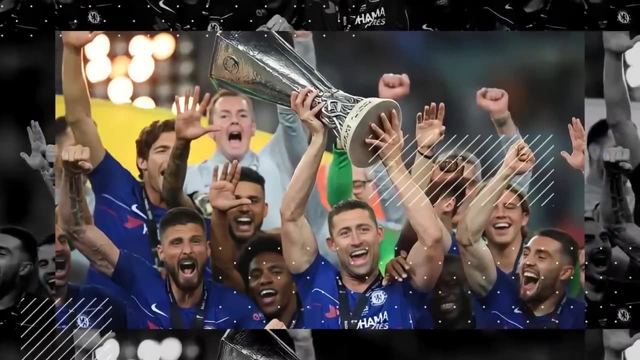 Okay, number 3. The UEFA Europa League trophy. Yeah, you heard that correctly. While the Champions League trophy is down in ninth place in our list of most expensive trophies, the Europa League trophy is up here in third, Without a shadow of a doubt. the Europa League. 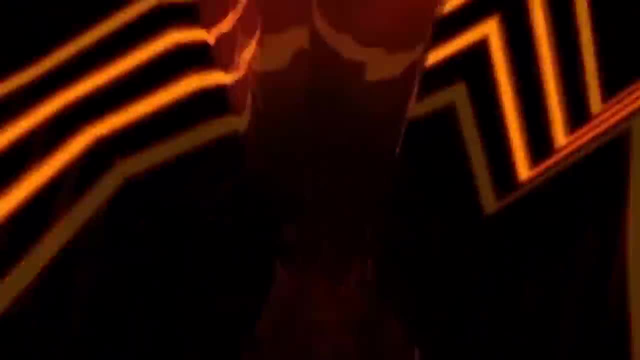 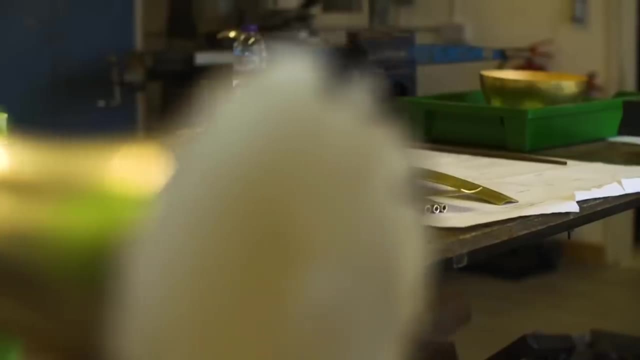 is the less prestigious of the two competitions, But the trophy that's handed out to the winners of that competition is 100 times more valuable than the big ears. The Europa League trophy is made of silver with a base of marble, and it is valued at $4.5 million.